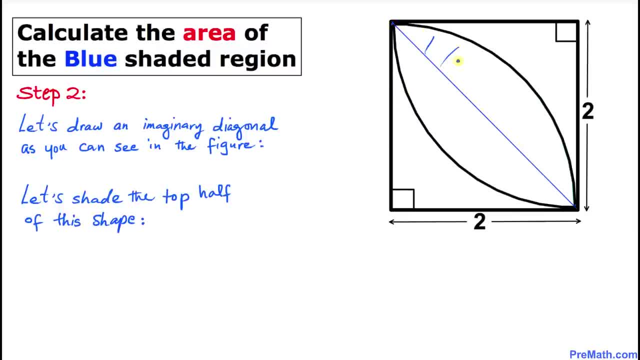 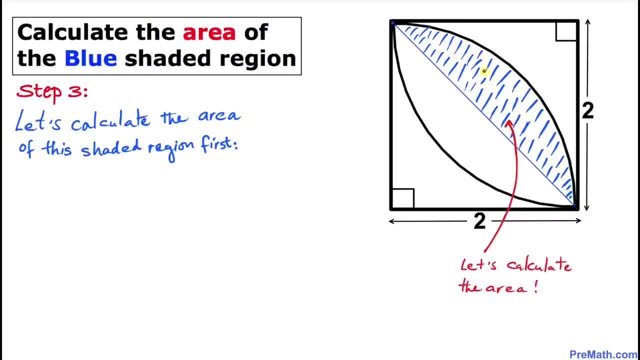 let's go ahead and shade this top half of this shape. and here is our next step. let's go ahead and shade this top half of this shape, this region, and now we are going to calculate the area of this shaded region first. now let's focus on 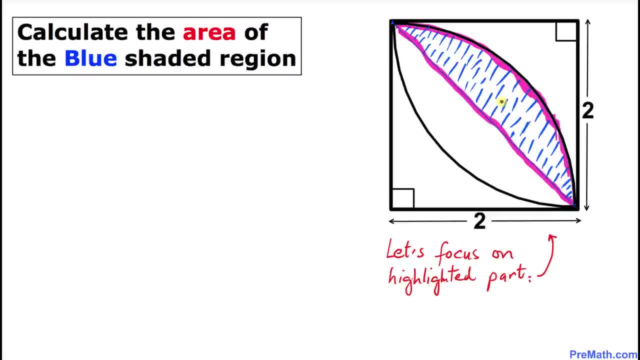 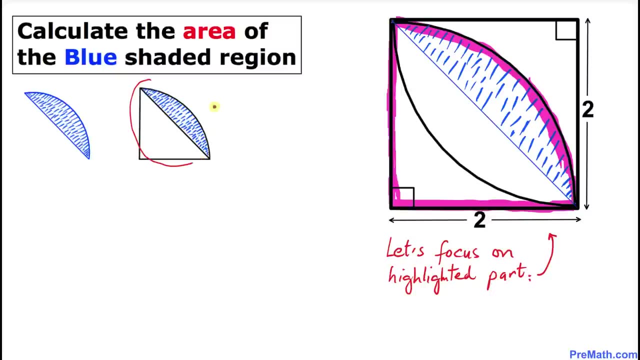 this highlighted part, and here I have nicely copied right over here. and now let's go ahead and focus on this highlighted part, and here I have copied it down right over here. and here is our next highlighted part, and here I have nicely copy it down over here. now let's focus on these three figures right over. 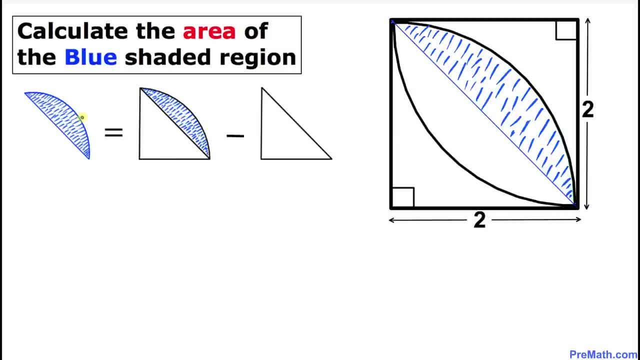 here we can easily see that this shaded area region is equal to this whole figure. govx म்' φ' थ त्रक्त दति, त्रक्त दति, त्रक्त दति. 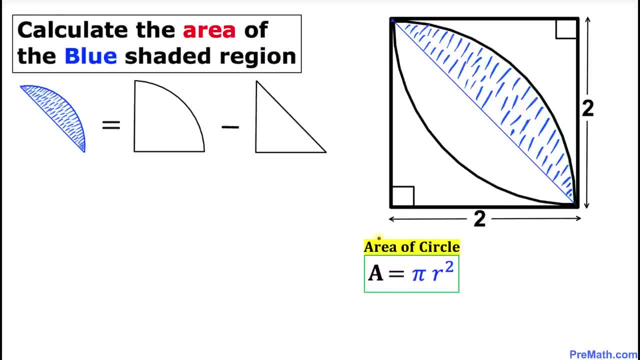 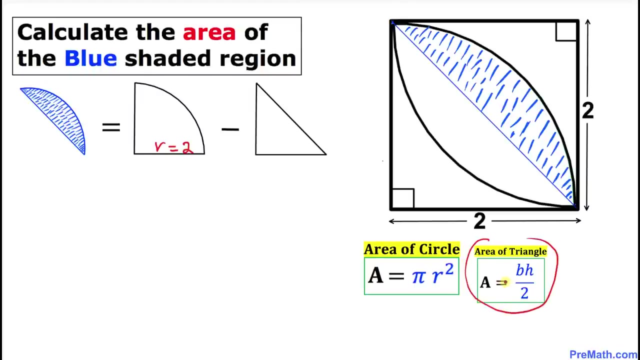 of this triangle. now let's recall the area of a circle, which is PI R square. in our case, radius R equals to 2 unit, as we can see over here, and the area of a triangle is equal to a half time base time height. in our case, over here, this 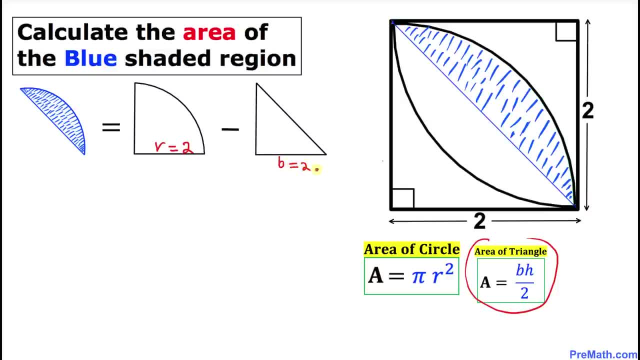 I'm going to call this base, which is 2 units- we can see over here- and the height is 2 units as well, as we can see over here. so the area of this region is going to be a simply the area of this quarter of a circle. 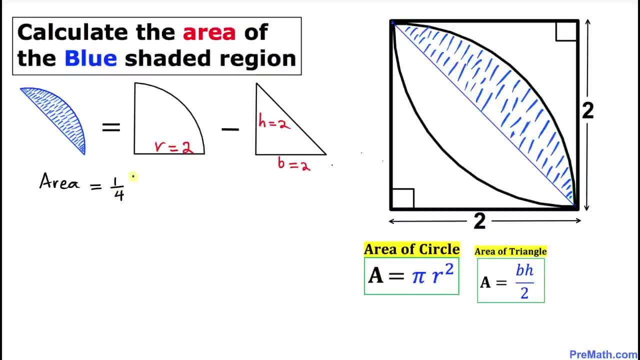 that means one-fourth times the area of a circle is PI R square. I can just write down: PI R square minus the area of this triangle is base times height divided by 2. now let's go ahead and fill in the blanks: one-fourth times pi. 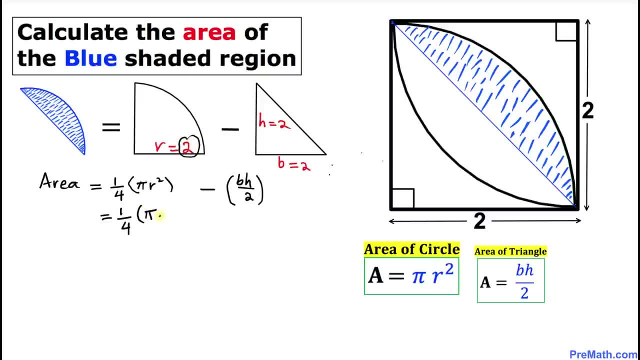 and in our case R is 2. so that is going to become 2. square minus base, in our case, is 2 and height is 2. so I'm going to put down 2 times 2 divided by 2. let's simplify further more. that is going to become 1- 4, and this is 2 square is 4 pi. 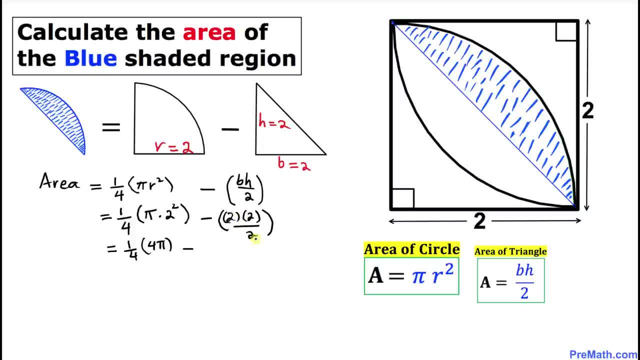 minus 5 2 times 2 is 4, 4 divided by 2 is going to be 2, so over here this 4 and 1 fourth cancels out, so we got pi minus 2.. So thus the area of this part this portion turns out to be: 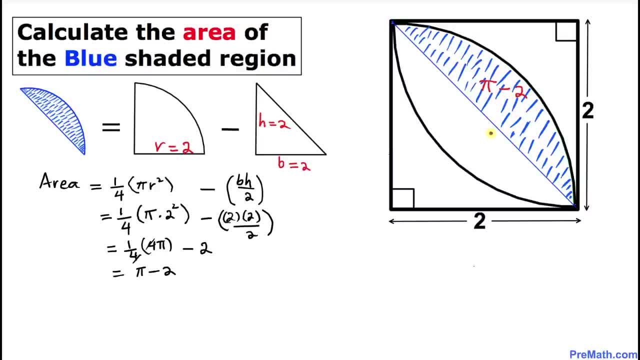 pi minus 2, and since these two parts are symmetric, they are the same, so we are going to multiply this thing by 2 to get the area of this full region. So thus the area of this full shaded region is going to be simply a equals to 2 times this. whatever area, we got pi minus 2,. 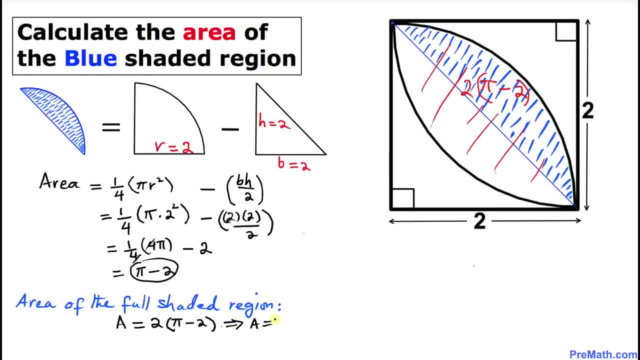 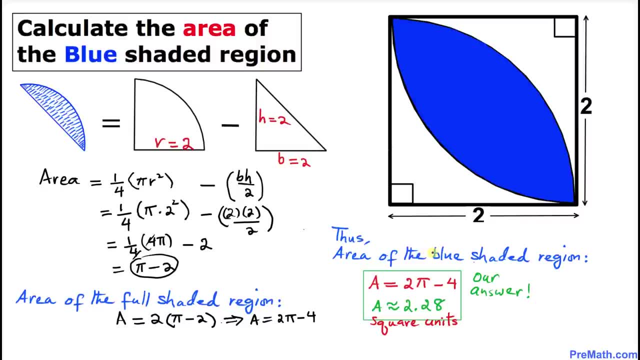 and that is going to give us a, a equals to 2 pi minus 4.. Thus, the area of this blue shaded region turns out to be a equals to 2 pi minus 4 are approximately equal to 2.28 square units. Thanks for watching, and. 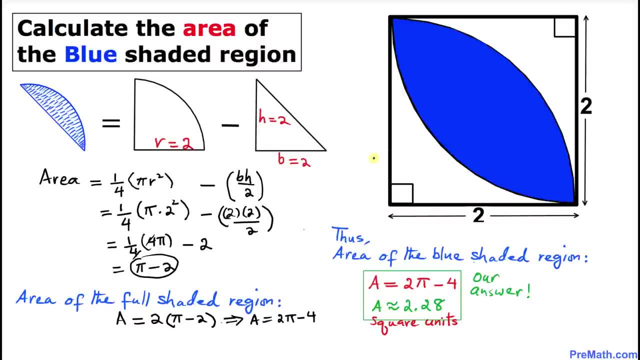 please don't forget to subscribe to my channel for more exciting videos. Bye. Subtitles by the Amaraorg community.